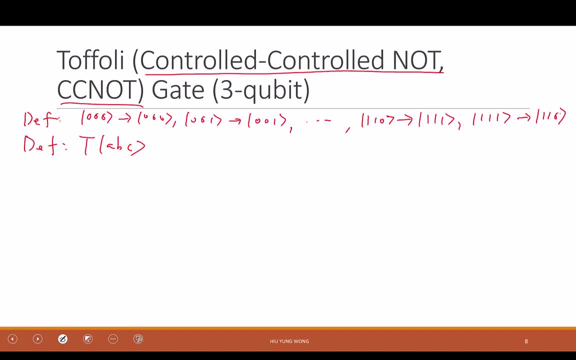 you said you can say happy or sad, doesn't have to be zero or one. okay, the definition is a b. i mean the, the, the final the. after you're applying the gate, it is a b and now i try to add the comma to make it clear. right, a b, c is clear. it has three. 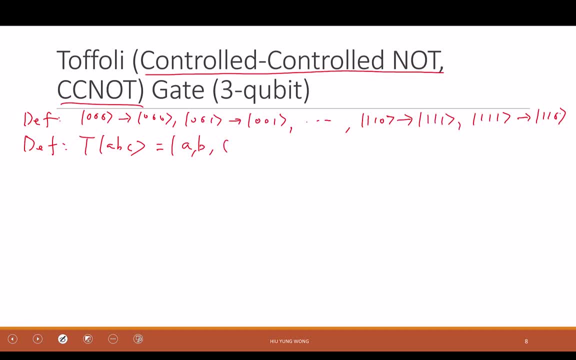 qubit. right now i make it clear, because i'm going to apply an equation a dot b, excuse of c, yes, exclusive. or let me remind you what is exclusive. or one more time what is exclusive, zero, exclusive or zero equal to what zero, zero, exclusive. or one equals to one one exclusive, zero equal to one, one exclusive. 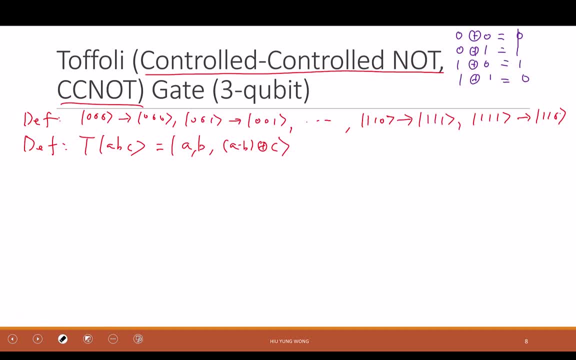 if one equals to zero, good. so let's take a look what happened. it's very interesting. if a dot b equals to zero, right here. dot is what n right? you change the n if it is equal to zero, then what do you got? you get zero, exclusive c, right. 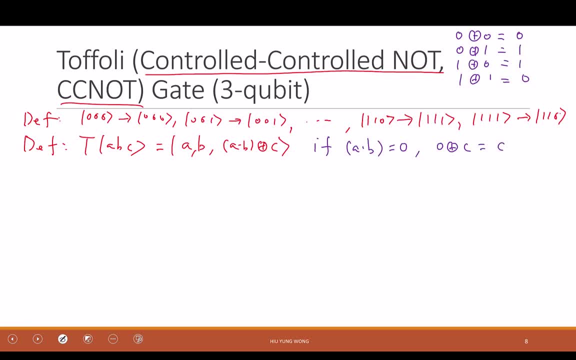 then it is c, it means unchanged, and that's why it's a control. control the a and b is. if any of the a and b is zero, then the whole thing unchanged. right, but what if a dot b equals to one? then you get what one exclusive zero. 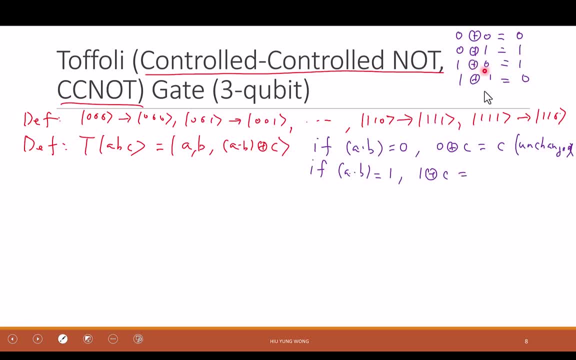 what is one exclusive zero? look at this. one exclusive one, one excursions, one equal to zero, and c can be zero or one right. this is just the lot of the c right. so this is what you learn in logic. if you don't know, i tell you. 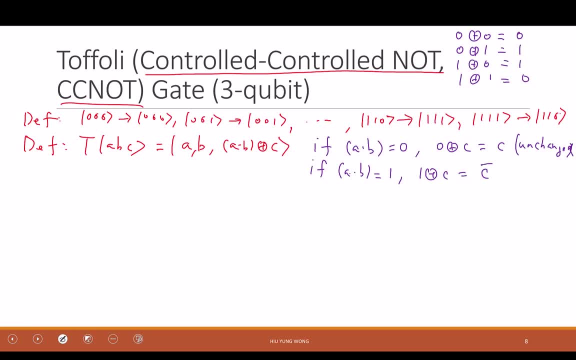 exclusive a bit. give you the knot of that bit that. i prove it to you already on top right. so you see that this is what? just a knot gate, but it's a classical knot gate, remember, okay, it's a knot gate. yeah, of course, a classical knot gate doesn't matter. the knot gates in the. 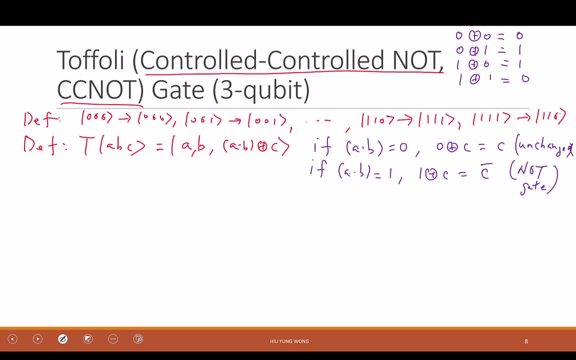 classical is the same as the knot gate in quantum for the basis state right if c equal to zero. what happened? a b zero equals to a, b, a dot b, exclusive zero right. if i apply the toffoli gate to a state which has c as zero, this is your a, b, a dot b, exclusive zero right. 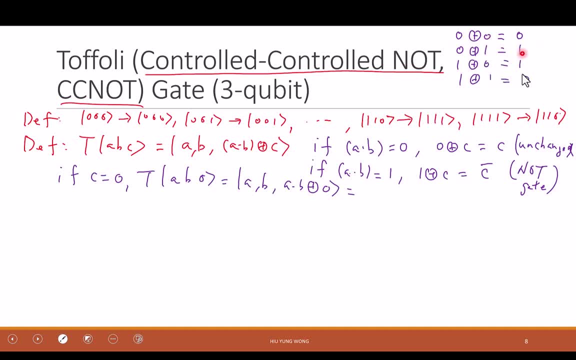 anything exclusive with zero is equal to itself. zero. exclusive zero, zero. one exclusive zero is zero, right? so it means this is equal to a, b, a dot b. what do you get? this is just a classical knot gate, right? so the interesting thing about toffoli gate is: 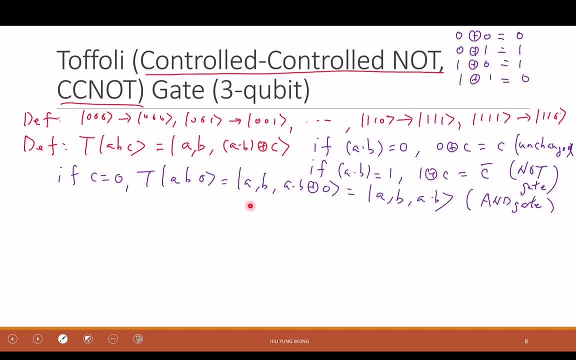 if you pick the input correctly, you can construct the end gate or not gate and you have learned digital logic before any gate. classical gate can be formed by the knot gate and the end gate. if you have a land gate, you can form any circuit. so it is a universal gate for a classical circuit. 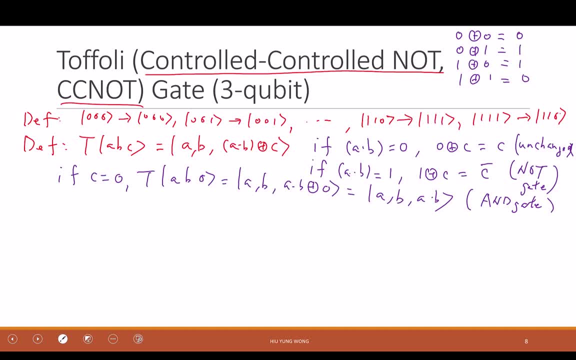 right? yeah, it's a quantum gate, but i told you, quantum gate is the same as a classical gate if we only consider the basis state, right? so this is uh toffoli gate. it can be used as the, so opening involved in the classic can. therefore can be used as: 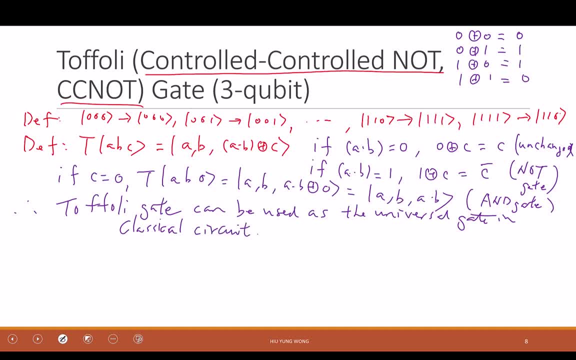 the universal gate in classical can therefore can be used as the universal gate in classical. so you, in principle, can transform the whole CPU in your computer to be just formed by Toffoli gate. that's the special thing about it, right? so? but but at this point I hope you can appreciate that the Toffoli gate is has effects, right? 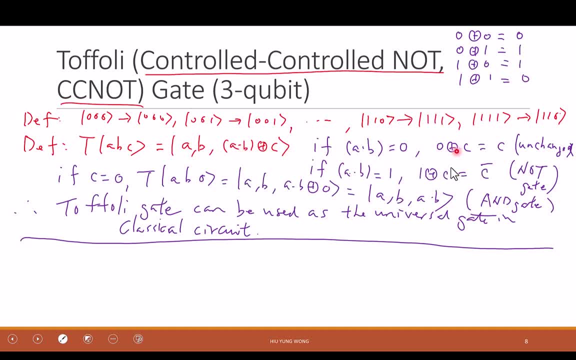 if A and B, they are, one of them is zero. C is unchanged, so you don't change the basis state until you have a one one zero, or one one one, until both A and B are equal to one. yeah, so I guess the last thing that you got is the Toffoli gate quantum. 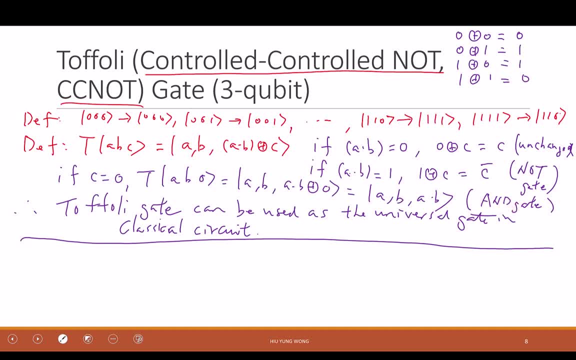 no, it's not an and that depends, yeah. yeah, I won't say that it's a land. I will say that you can be use it as a north gate or land gate. then you have multiple portfolio gate, then you can form it. then, of course, you can form the land. 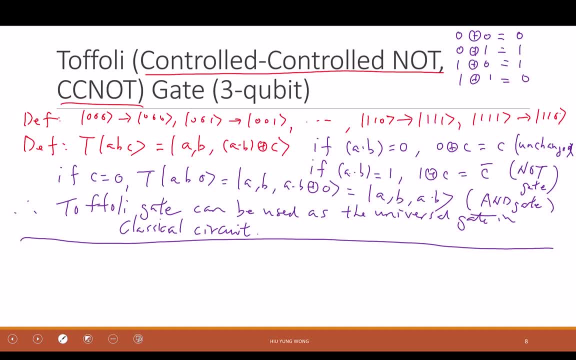 right, as I have a north, you have, and then you can form any type of gate in classical circuits, yeah, but you cannot have the land gate at the same time. you need two portfolio gate right. one of them, you put the input AB equal to one, then you get a north gate. another, you put: 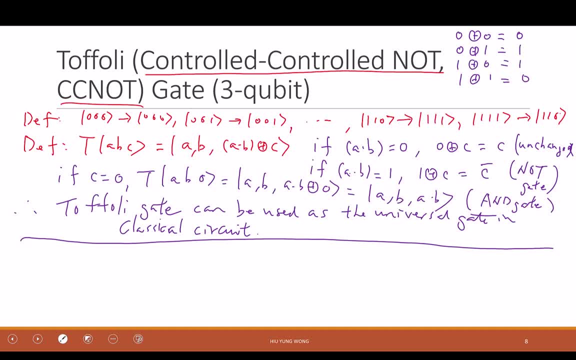 a C equal to zero, then you get a land gate. then both of them becomes a land gate universal. it means you can form anything by using a portfolio gate. yeah, so can you guess what the matrix look like? eight by eight? very good, right? the first thing is the size. 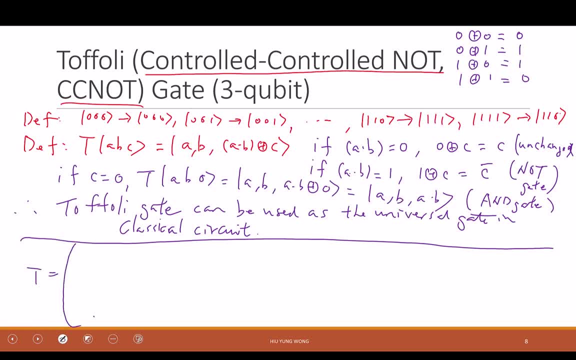 why is eight by eight? because it is three qubits. so two to the power, three right and then, based on what we have discussed, can you guess? one zero, zero, zero, zero, zero, zero. a lot of writing. I suggest you not to write it, only I write it right. 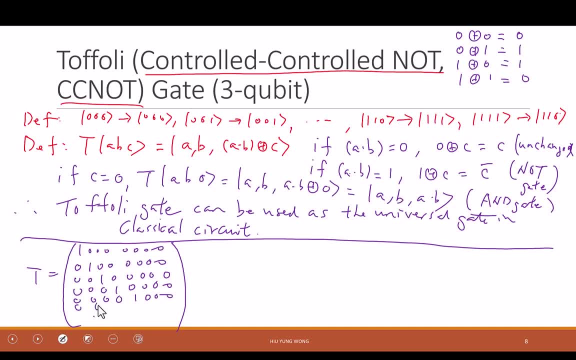 it's all diagonal at the beginning until the last two it becomes a north gate right, and we understand the reason we do this is because this row- and I will explain you in the next slide- actually let's do some uh exercise right. for example, if t times 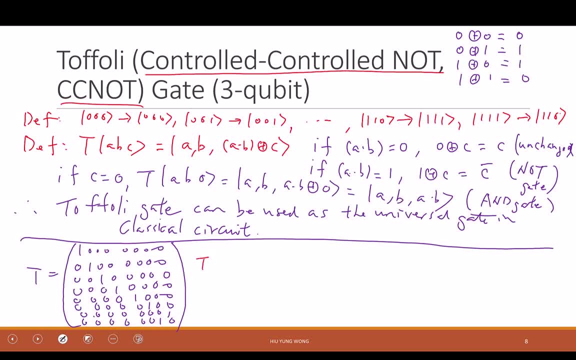 right. for example, if t times right. for example, if t times 2110, what does it look like? you will be able to write: so, one zero, and then eight by eight, one zero, but no, and then you can also write 0, 0, 0, 0, 0, then C into 4. 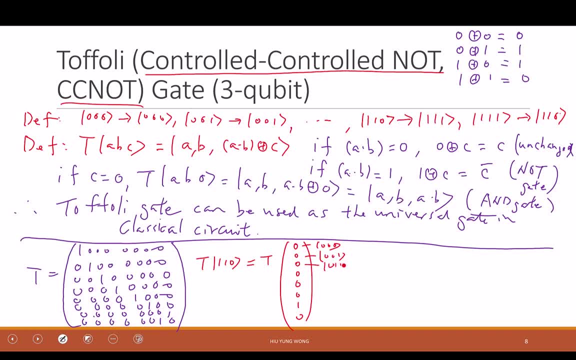 0, 5 single C 0 5 money will be therecipated line and so it get's only about 0, 1, 0, 1, 0, all the way. here I have one component of 1, 1, 0, zero component of 1, 1, 1, is that clear? 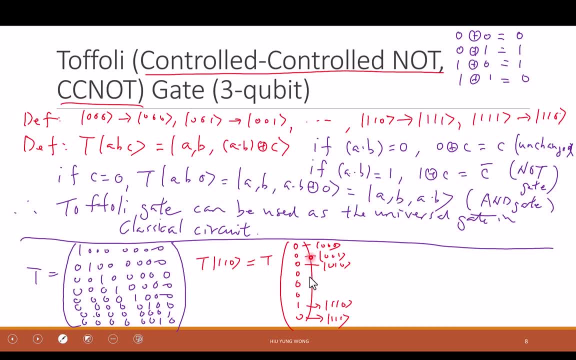 Now, there I do a multiplication, not difficult, right: T times this one column times row times column. what do I get? This one column times row, I mean row times column. what do I get? Zero, right. 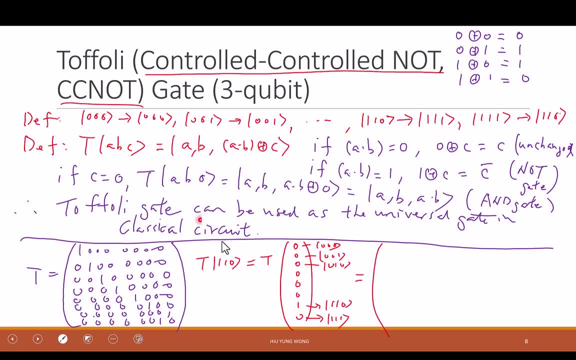 Because you multiply this first element by this first element plus this element, plus this element, you only get long zero if the corresponding part, both are zero, right? This one has the first one, 1, and this is zero. no way right. 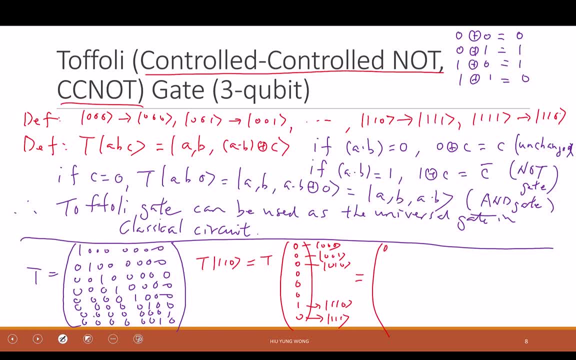 So that's why I get zero for the first one. second is also zero because the second one is the second one is 1, but here is still, the seventh is 1, right? So I keep doing So, I keep doing this and eventually I find that 1,, 2,, 3, 4, 5, 6, 7, only the last row I have, the seventh element is 1, and this is seventh element is 1, right. 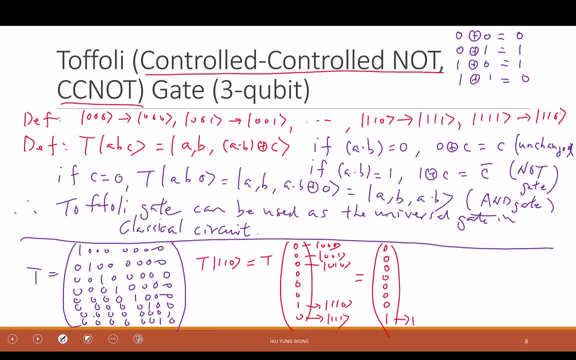 That's why it achieved the purpose of making this one component of 1, 1, 1.. Is this okay? Anyone clear? Any questions? Any questions? Yeah, I don't know. Okay, this is not gay, right. 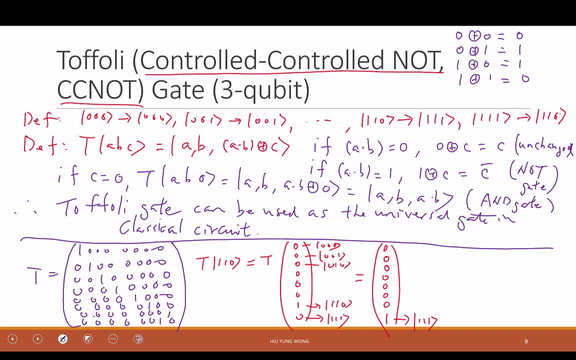 So it's not secret. It's not a secret, It will be. what does C get? 1, negative, 1. Bigger, bigger. I'm a control, control, phase shift gate in plus, minus basis. So it's also like there's phase shift, phase shift, phase shift. 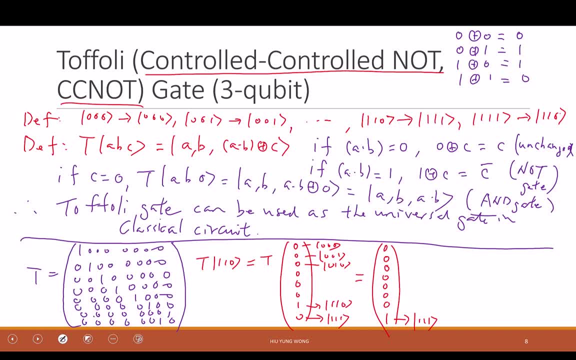 Only not general phase shift, but the C yeah phase shift: 100 degrees, 180 degrees. Yeah, you're right, That's what we said earlier. Now you can try. I never try, I never really read it or try, but that's what I guess, right. 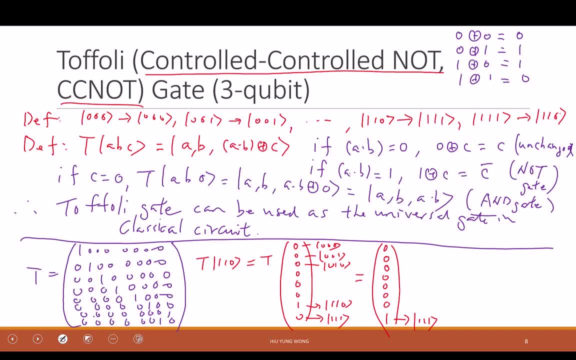 We can make them as the in the midterm. You just try to prove it. Okay, everyone try it. okay, Any questions? Someone still puzzle? have some puzzle? Is it clear? Yeah, Now do you need to play with the matrix to have? 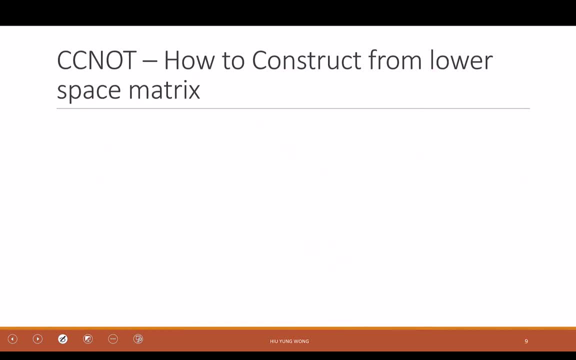 to have a deeper understanding, right? So I assume you're okay. Now I want to go over this on how to construct a matrix. Why am I losing one slide? Oh, okay, I have two slides Now. C-lock gate right. 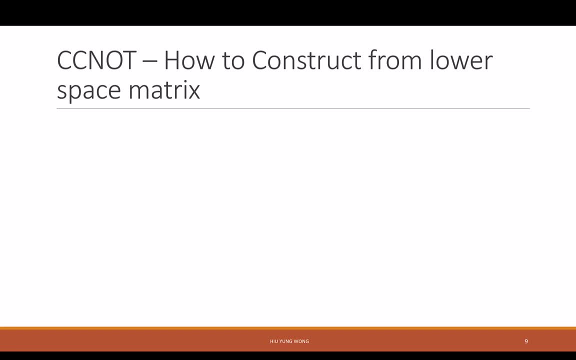 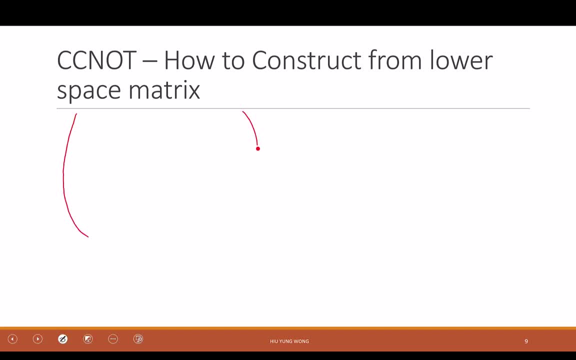 and actually I won't mention everything, I will just make this simple. Let me write down the matrix one more time of this top polygate. okay, One-zero-zero-zero-zero-zero-zero-zero-zero- one-zero-zero-zero- zero-zero- zero- zero-. 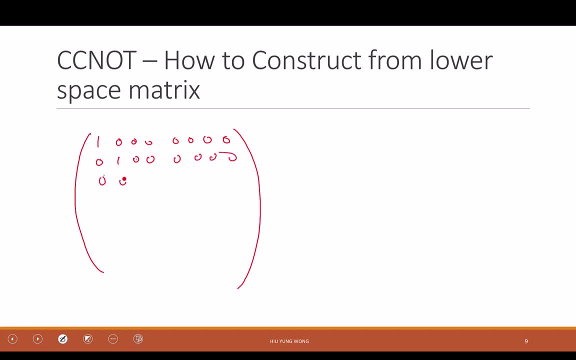 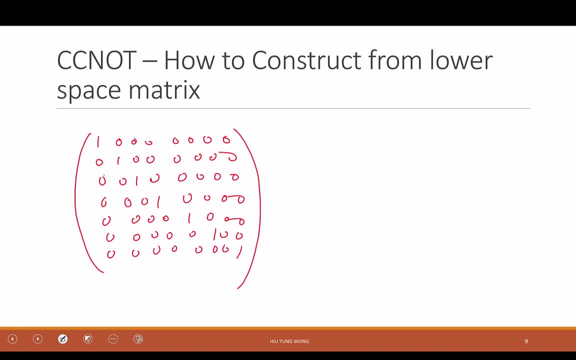 right, zero, zero, one, zero, one, zero. okay, what does it mean actually for each column? for each column, you think about this- when you do a multiplication on a vector- a 0, a 1, a 2, a 3, a 4, a 5, a 6, a 7 this one is referring to- I have a 0. 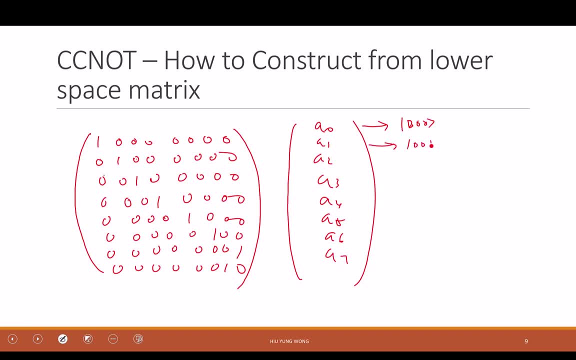 component of zero, zero, zero, zero one, zero, zero, zero one, zero one, zero one one one. zero, zero one, zero one one one, zero one one one. is that okay? what does it? do you actually? this one is going to be take the. how much is going to multiply to the components of zero, zero. this one multiply the component of zero, zero one. 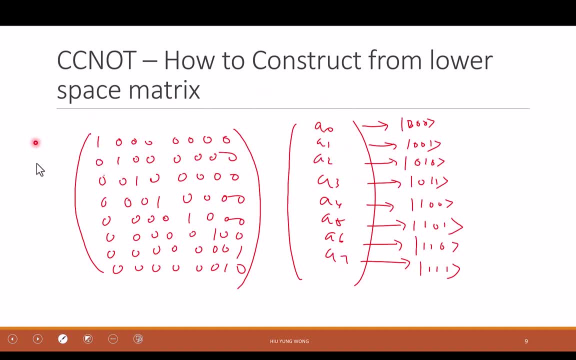 right. and then the whole thing you add together, it becomes zero, zero, zero. so in this one, basically, in each element t i j, row and column right is actually equal to i t j right. so this one j, as i told you earlier, it's just a sandwich of this product, right? it's telling you that. 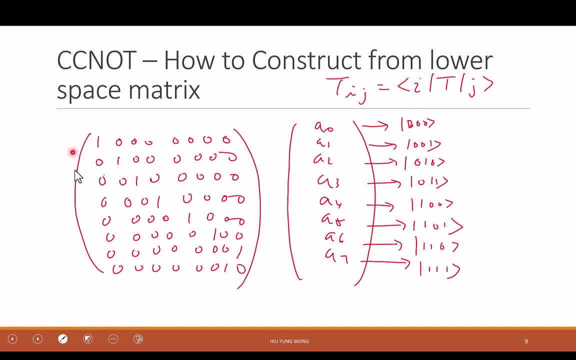 how much in order to have the after rotation to have the i component is telling you how much of the j component of the input vector will contribute. so basically, in this matrix you can cheat the row as now. i'm going to make it simple. i'm going to change it to: oh. 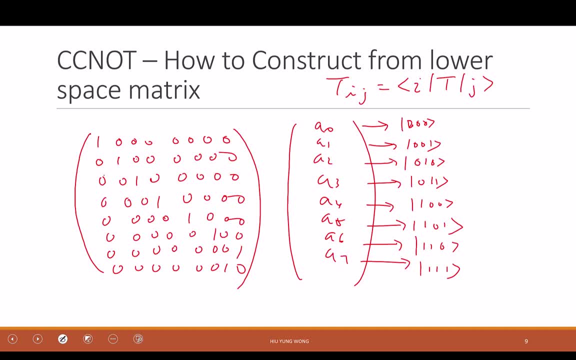 no, i cannot, because i want to show you something. I still use the. the binary. this is 0 0 0 0 0, 1 0, 1 0 0, 1 1 1 0 0, 1 0, 1 1 1 0, 1 1 1. this row representing 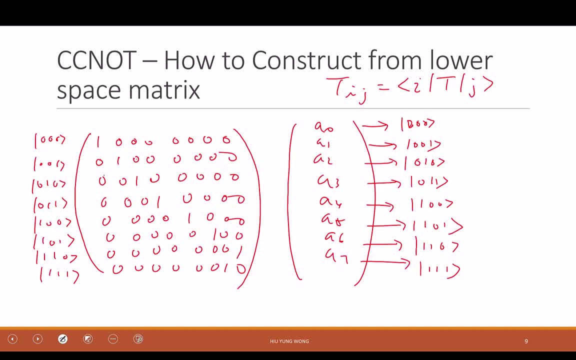 after multiplication, where these elements will go to. they are going to contribute to the coefficient of this final state, right. and then on the top, this one is representing what it is going to. how do I say overlap with right? right, 1 0, 0, 1 0, 1, 1, 1, 0, 1, 1 1. yeah, say louder. last second row, which one? this? 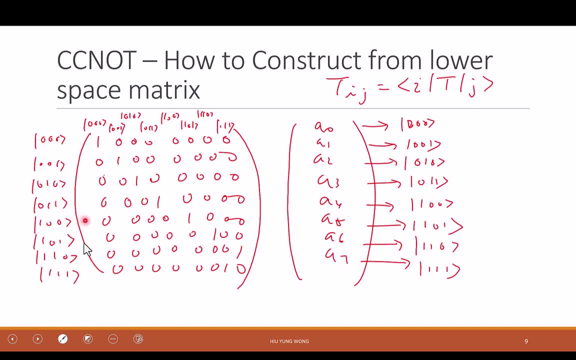 one: 1 0 0, 1 0 1. are you talking about this? so 1 0 0, 1 0 1? oh, this row is for 1 1 1. okay, what should be the value of this one? 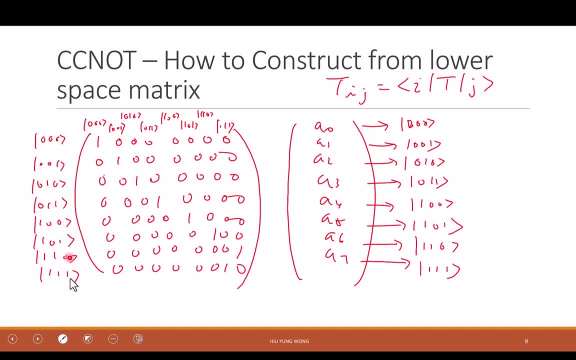 1, 5 rest: 10, 15, 16, 17, 18. I think that's the max. you don't have to do 100 English. you don't have to do American English after to get your job done. so what, what? what's wrong? Oh no, no. matrix has nothing to do with the content. this row represent how. much you contribute. for example, when you do this multiplication right, this row multiplied this row give you the components for 1, 1, 1, correct? How do you get the output of this one? This row multiplied this row give you the Kara. what's wrong? 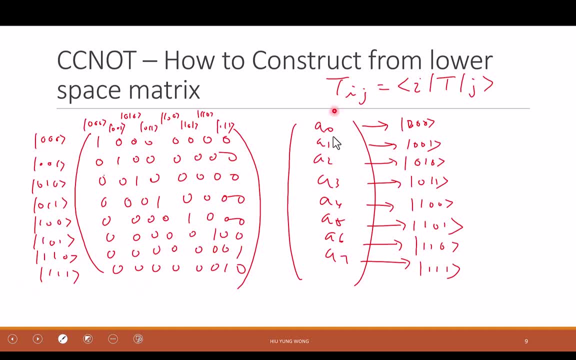 components for 1, 1, 1. correct mod. Empress rationals of this Row. Multiplied this row give you the components for 1, 1, 1. correct one one: this row. multiply this column give you the components of one one, zero. that is how you do matrix multiplication, right. 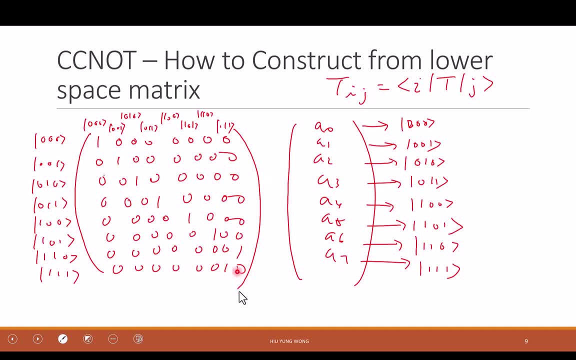 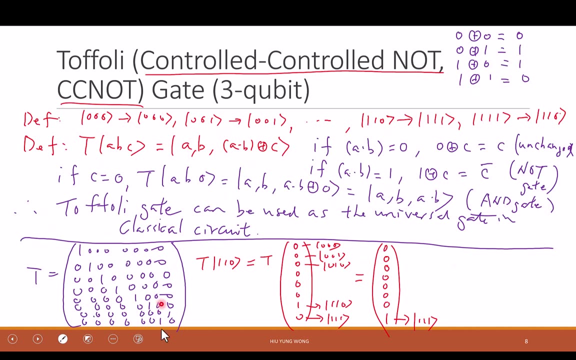 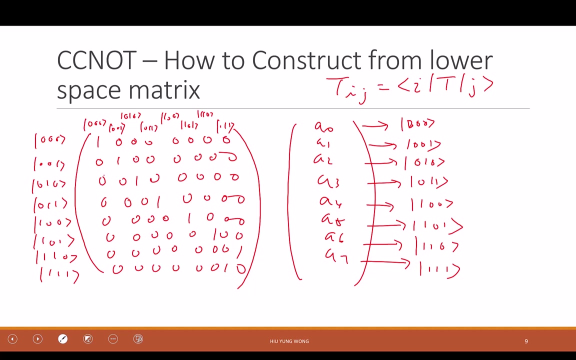 last. so this one? no, because this is t matrix. this is not identity matrix. the t matrix is zero. one one, zero. this is the toffoli gate control knob gate. right, if this is one one, there is identity matrix. this one, okay, yeah, yes, yeah, i'm trying to tell you that how to read this matrix, because i 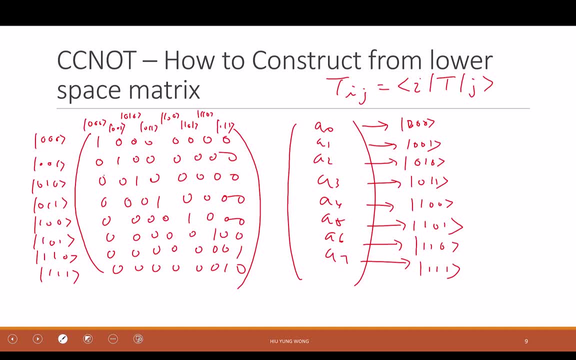 want to construct from a lower space, but we, you know that already, but i want to show you one more time, uh, how to do matrix multiplication. when you do matrix multiplication, you do this row times, this column. what does it mean for each of this element? it means how much component, how much? 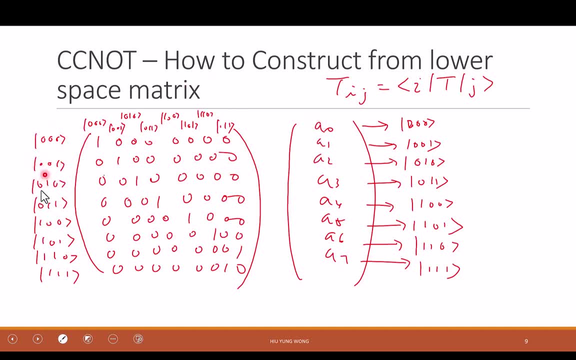 overlap of this final right. each row. give you the fine, the, the component of the final basis vector: zero, zero to one one, one right. because this row times this column, give you the component of zero, zero. correct this: one times this column. give you component of this column right. the last row times this one: give you the components of one. 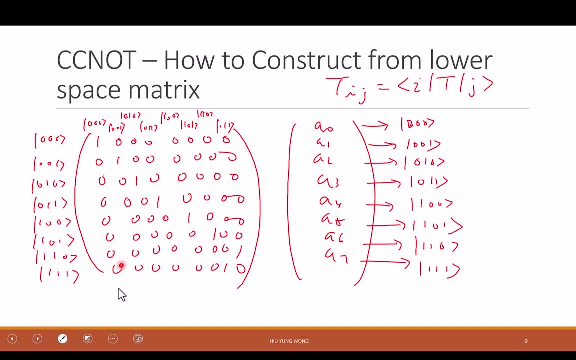 one one right now. and then, for each of this, actually, it tell you that how much come from zero, zero, zero. how much come from zero, zero, one. how much come from zero, one, zero when you do the multiplication. okay, so now, if you look this carefully, you see that 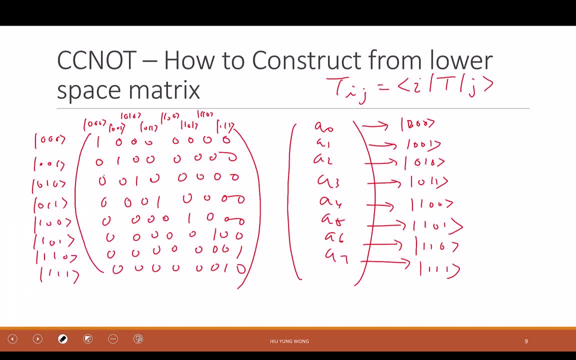 if i become, i can cut this into this. when i cut into this, what's so special? look at the first one, the most significant bit. they are all zero here. the most significant bit: zero, zero, zero, zero, one, one, one one. do you see that right? so that is how the matrix work, right? the most significant bit. 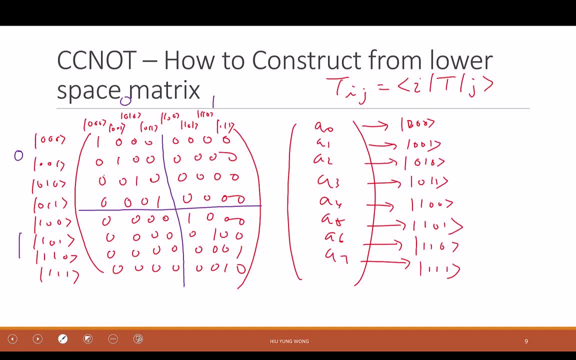 the, the, the most relevant gates can be decomposed in this way. right, so this is uh, i call it m s b now. then let's continue to decompose it. i will only decompose a to the second most significant bit. right, look at this isn't, this is zero. 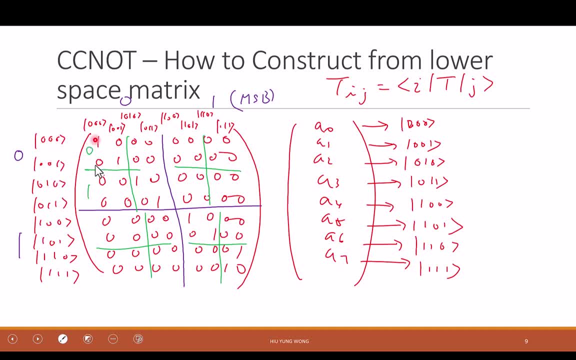 one for the second most significant bit: zero, zero. they are all zero, these are all zero right. this is one, one right. but for the here is zero and this is one right. for example, these four, they both have the second bit one one and the second bit one one. 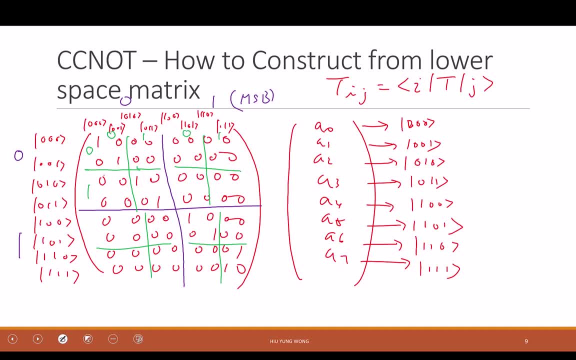 right, so same here: zero one, zero one, zero one. no, zero, zero one, one, zero one, one, zero. right again, for example, this block. i have the least, the second most significant bit: they are all one, because they're zero one, zero, zero one. they're all one. and here they're all zero. for the second bit: 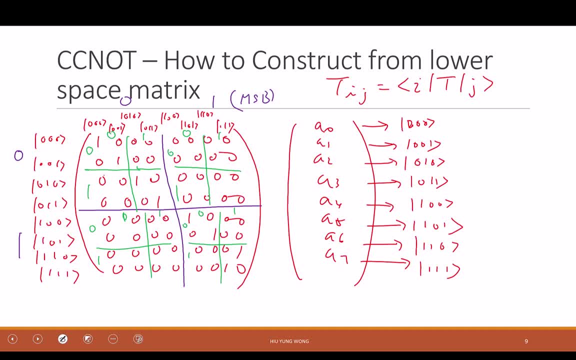 right? so that is how it is constructed. um, so the green is the second bit, right? so i i won't continue. if you continue to cut it, then you will see the third bit will just keep cutting right, and so you. you see that, in order to construct this, 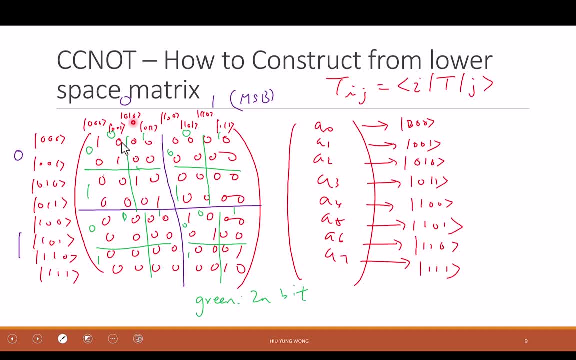 bit. you will see that this part is the identity, right, and it is identity when the first bit are all zero, right, and then for the second part, this is: uh, it's zero, is nothing, everything is zero. i can ignore it. what is this gate if this is two qubits? 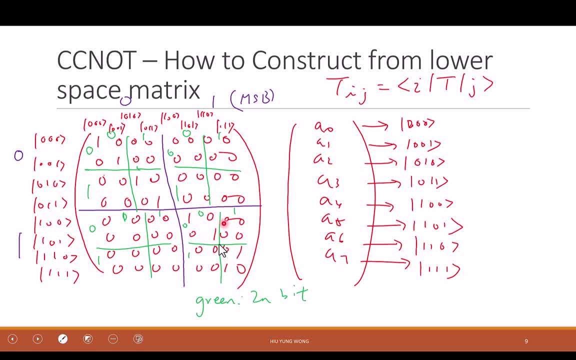 is it only or exclusive or right, control, not gate, right, let me write it verbally: which color to use this block? this block is a key part of the block, the one and the other block. i will say so, i will say this part right, the one and the other. 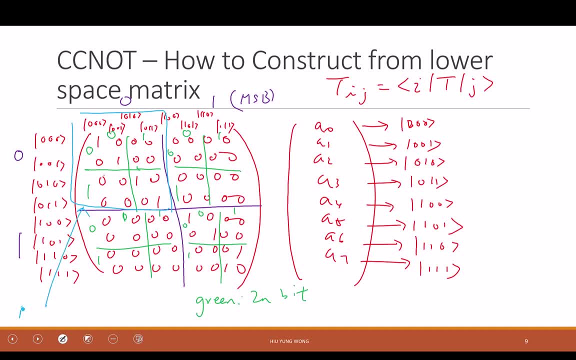 block when m s b 0: 0. the one and the other block. block the one and the other, block the rest is. i okay this block when m s b is one. the rest is control. not that's what i want to say, right, it's not easy, this one, uh, also took me a long time to understand, right, but i want you. 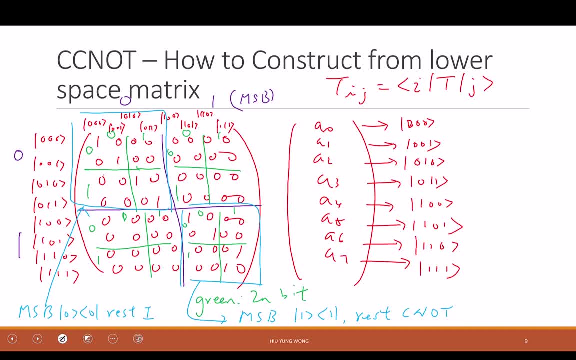 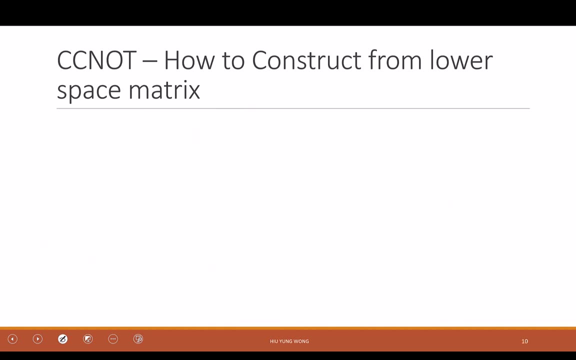 i don't need you to decompose to this way, but my approach is: you trust me, i give you the equation. in the future, you use similar approach. when you do that, you try to construct it, to verify, make sure you get the right answer if you are not clear. so, by doing all this, that's what i say. 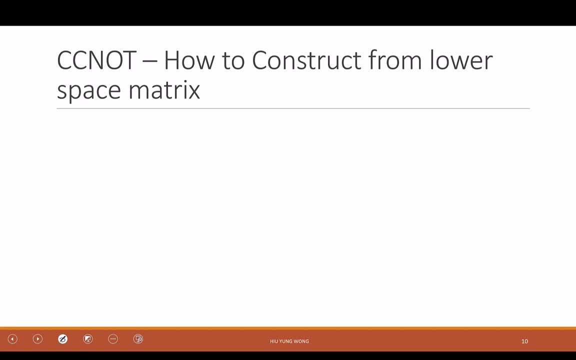 how do i construct the matrix? i can say that this is equals to the t gate, equals to when i write zero, zero. this is the first bit. this is the m? s b right, the left, one tensor product, the identity matrix, but it is the two qubit identity matrix. 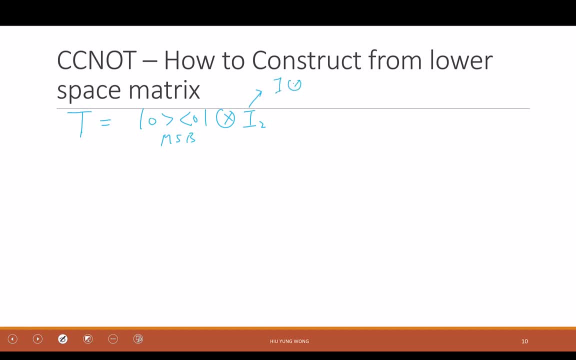 okay. or this is i tensor product, i okay. plus, when it is one one, it is the c naught gate for the two qubit. okay, let me finish this. then maybe you'll ask: first, is there a methodical way? i see how you started partitioning the matrix and then kind of guess. 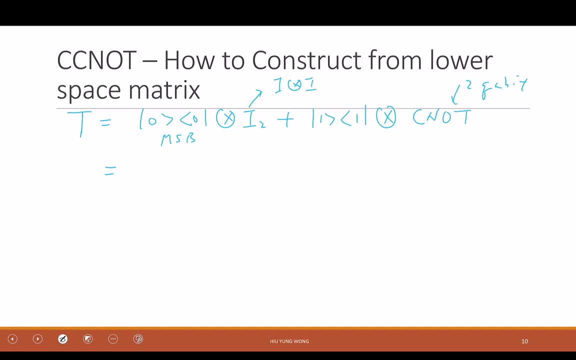 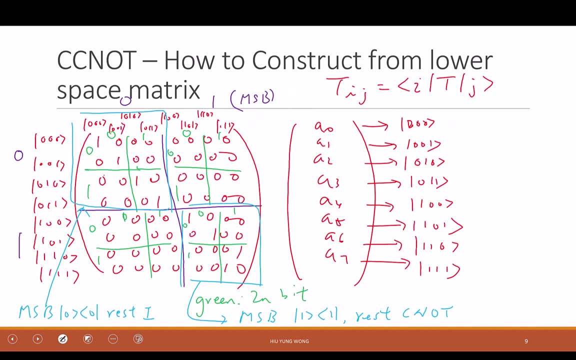 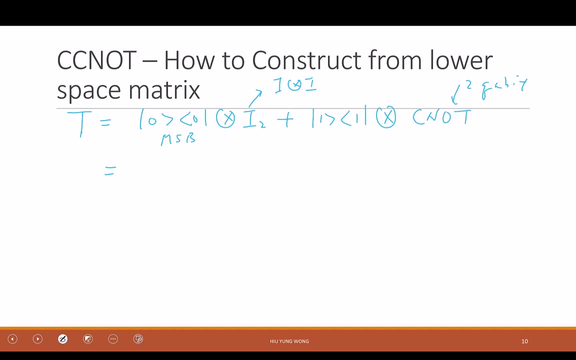 to arrive at the matrix, right. so how do you think we lange you or not? you know, through the systems. for example, if i give you the matrix, this is the only way you can do that right. i'm doing it based on matrix, but you you can have other understanding. for example, you know this is a control control. 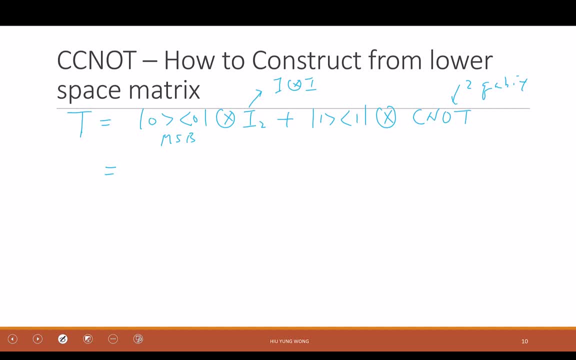 node gate, then you already know that if the first qubit is zero, i should have an identity, because it's ctrl, ctrl, not right, and then the sec, the second one, it should be ctrl, xe, not. first qubit is 1, then it must be a control knob. think about that, let me. 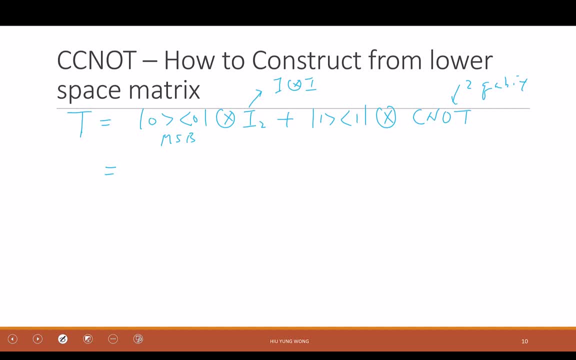 show this first. okay, so what is 0? what is this in column form? huh, 1, 0. how about this one? 1, 0, right. what is the matrix form of a 2 qubit gate? identity gate: 1, 0, 0, 0, 0. okay, good, how about the second one? what is that? oh, I need to. 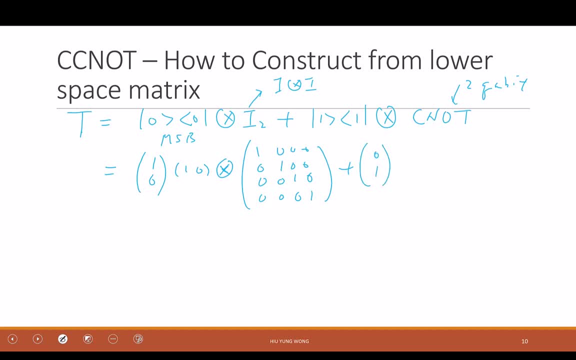 wrap up quick. okay, so this is 0 1 0, 1 control knob. you already know: 1 0, 0, 0 0, 1 0, 0, 0, 0 0 0, 1 0, 0, 1 0 right. 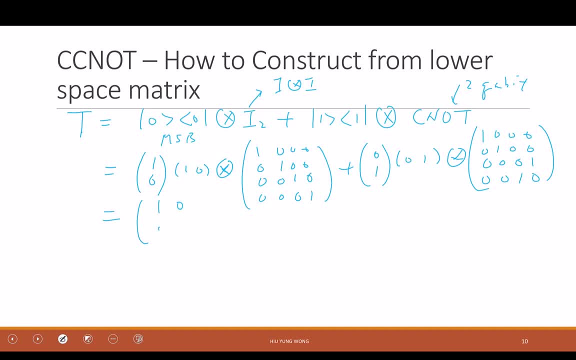 I just redo this. this is 1, 0, 0, 0. do you see that right? I just do the whole thing to save time. 0, 0, 0, 1. okay, so if I put this in: